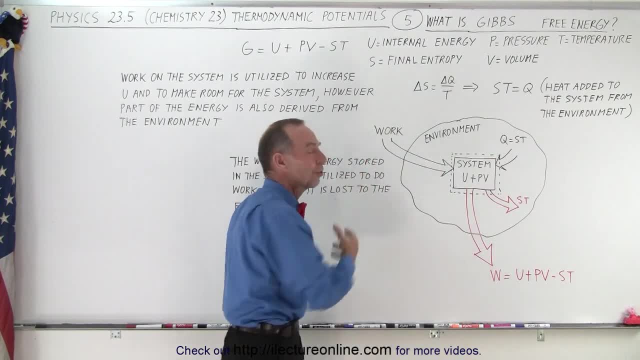 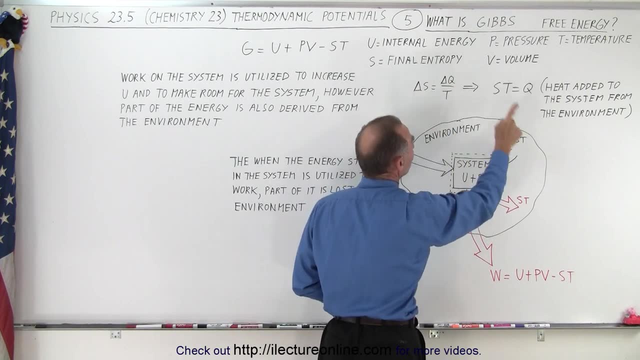 from within the environment, and we call that Q the heat added to the system from the environment, and Q is equal to s times T, where s is what we call the final entropy and and t is called the temperature. now, without knowing too much about entropy at this point, 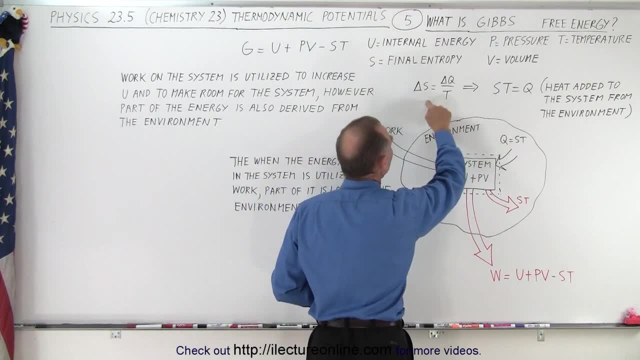 because we have to go look at some other videos to do so. we can go here and realize that the change in entropy of a system or of the environment and the system is equal to the heat exchanged divided by the temperature which it happens, and that means we can rearrange the equation. 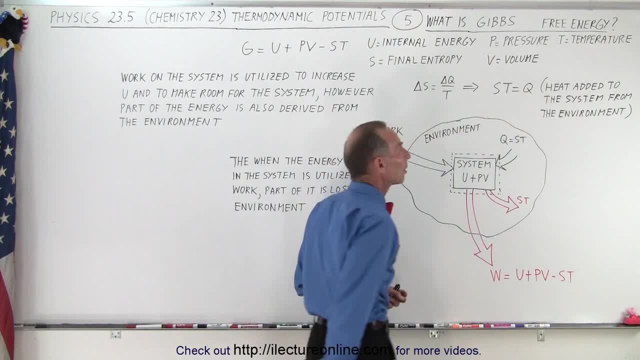 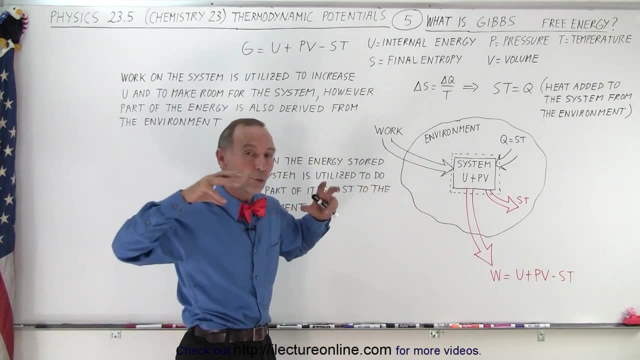 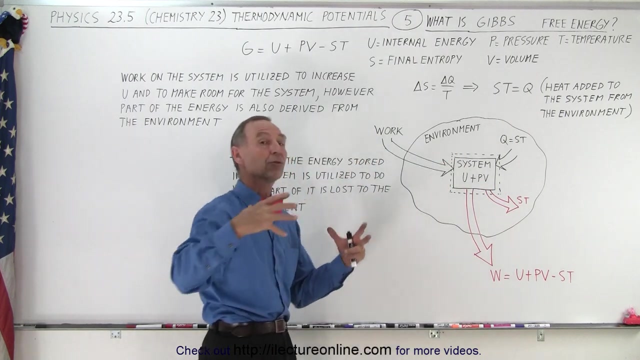 and show that s times t is indeed equal to q, the heat added to the system from the environment. so when we add heat from the environment and we do work on the system, all that together does indeed increase internal energy and it makes room for the system. now, when we go back and try to 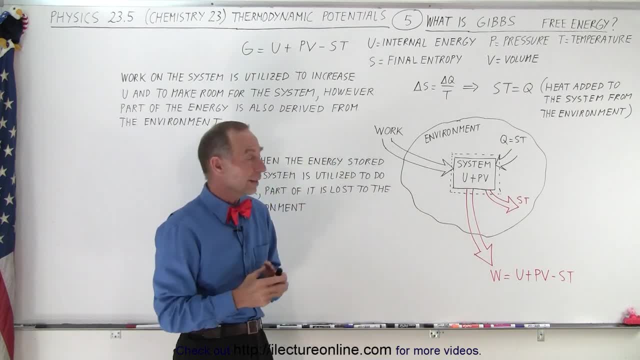 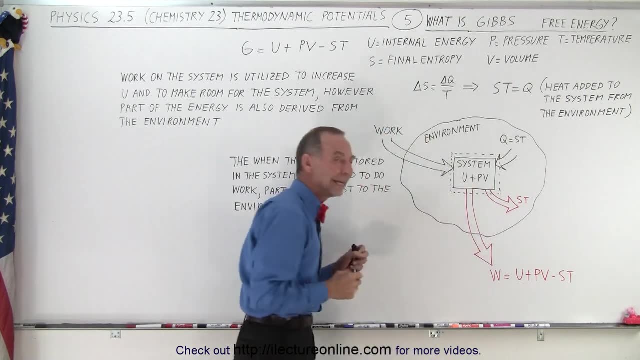 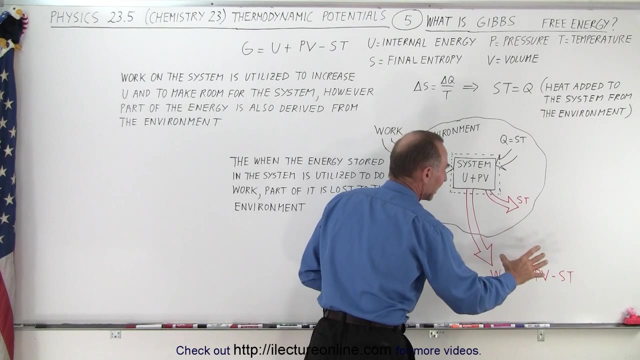 reutilize that energy to do work well. unfortunately, not all of the internal energy and not all of the energy stored, as the increase in volume, can be utilized to do work. some of it is going to be lost to the environment and it's the total amount of energy available from internal energy plus the 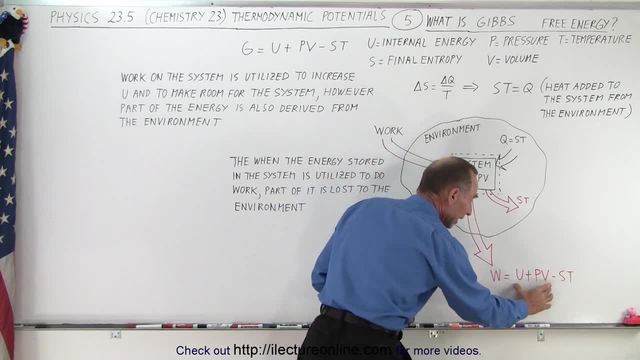 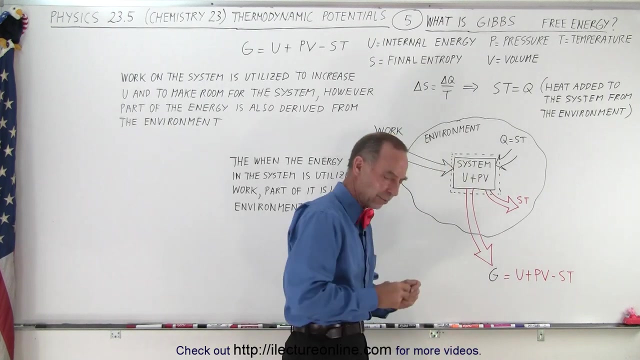 volume, the energy stored in the expansion of the volume. we take all that energy. we subtract from that the energy loss to the energy. oh, and wait a minute, this is the wrong symbol here, isn't it? yes, here i need gibbous free energy, so i need g, not w. oh, no, actually. no, that was right, i'll go back. 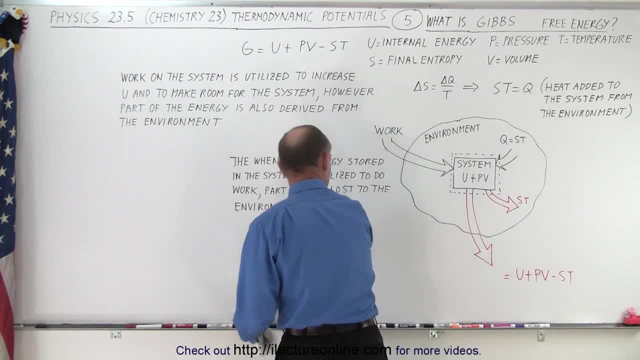 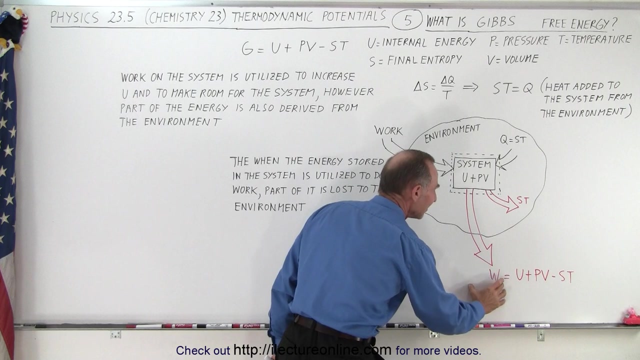 i shouldn't have done that. ah, all of a sudden i realize no, that is indeed w the work done. so let me repeat myself, because i think i for a moment there had a brain miss, a malfunction, so to speak. but anyway, the amount of work that can be done is not equal to the total internal energy plus the energy stored. 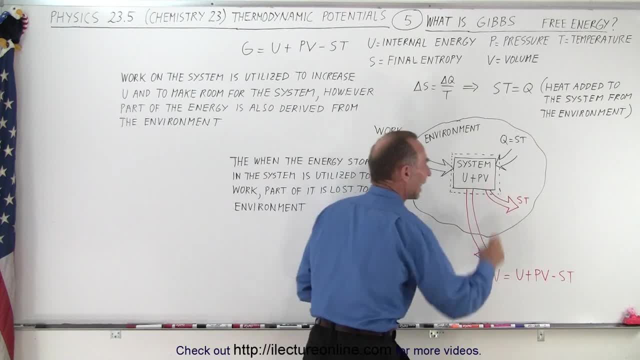 in the expansion of the system, some of it is lost and is absorbed by the system. so the amount of work that we can do is actually less than the available energy, and that work that we can do is not equal to the total internal energy plus the energy stored in the expansion of the system. 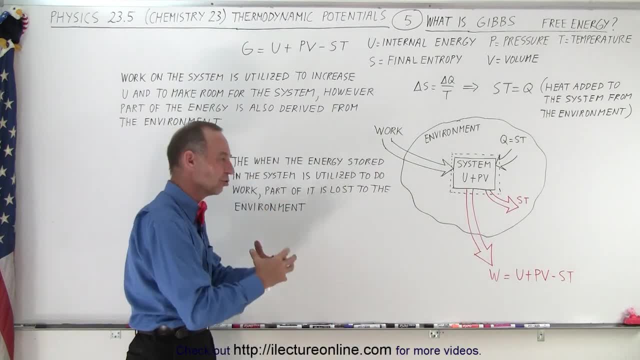 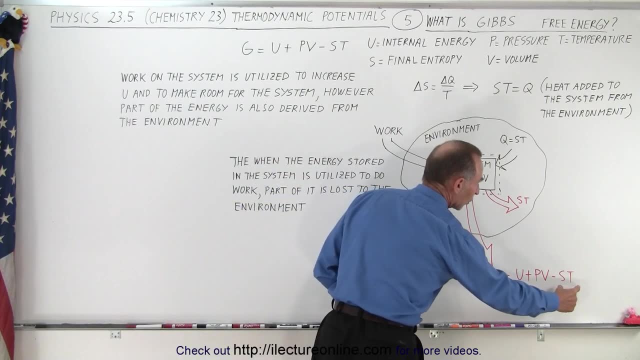 so the amount of work that can be done is essentially equal to the gibbs free energy. that's the definition of the gibbs free energy. it's the amount of energy available to do the work. because we can't utilize all of it, we're going to lose some of it to the environment, and so when we put 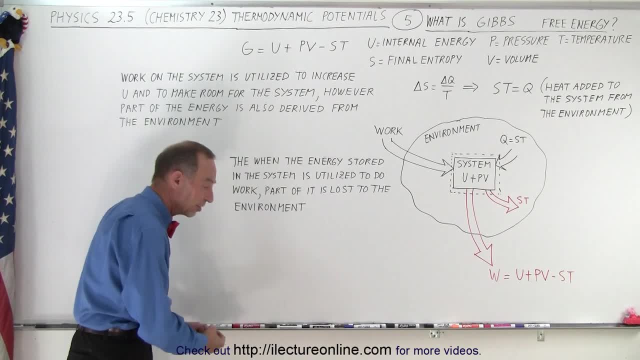 energy into the system, we get some energy from the environment. when we pull energy out, we give some of the energy back to the environment. so here, when the energy is stored in the system, when the energy stored in the system is utilized to do the work, part of it is lost to. 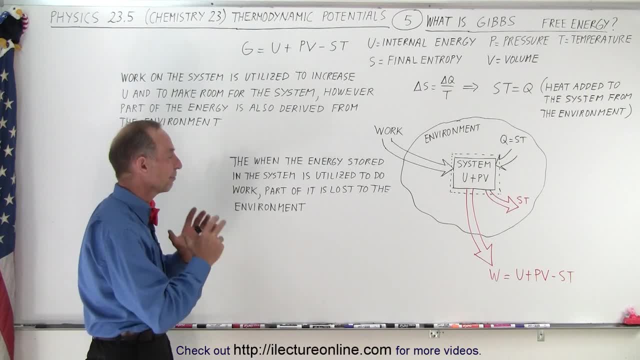 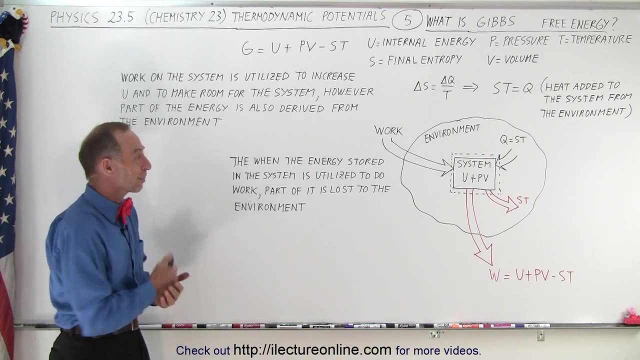 environment, and so that remainder of the energy that's available to do work is called the gibbs free energy. and that is the final of the four thermodynamic potentials. now that we understand them, at least from a top level, we're going to dig in a little bit more and see how they're utilized. 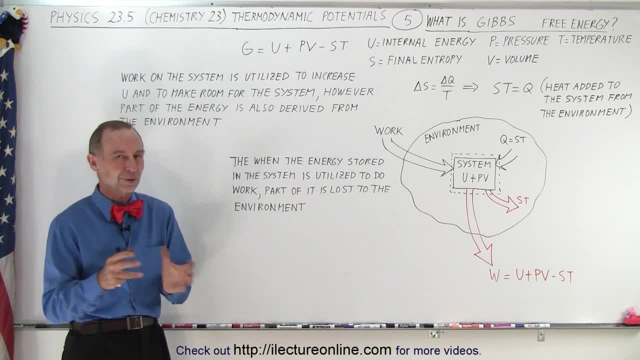 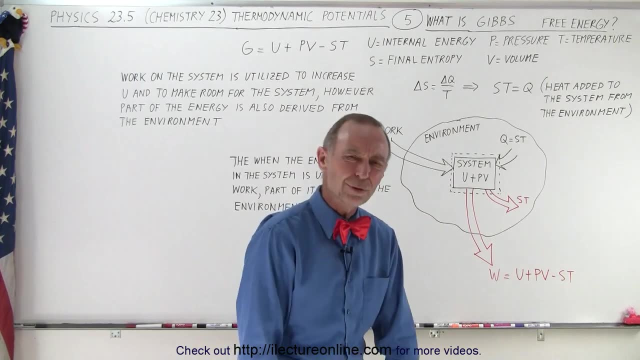 and how they stack up against one another. so stay tuned and we'll show you some more details and then, eventually, some examples of how to actually utilize these, especially when it comes to enthalpy. so redo that one. no, you're good, all right. 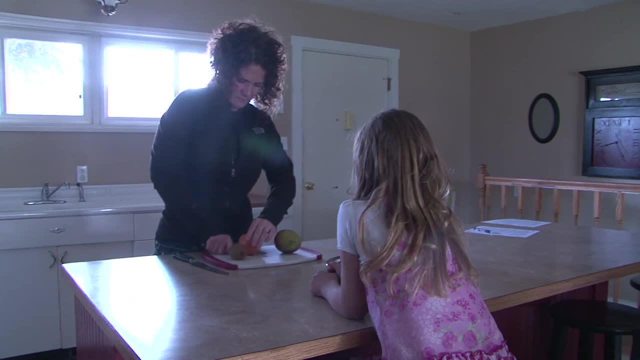 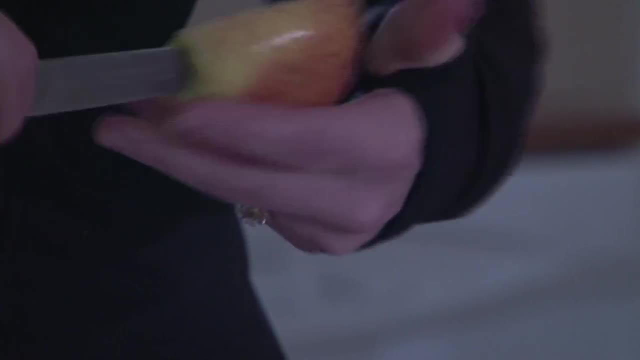 Spending time with your kids in the kitchen can make for fun family memories. It's also a great way to get a little help with household chores. But the kitchen is also full of potential hazards that everyone needs to be aware of. Tiffany Egan and her daughter Sadie learned that lesson while working together in the kitchen.